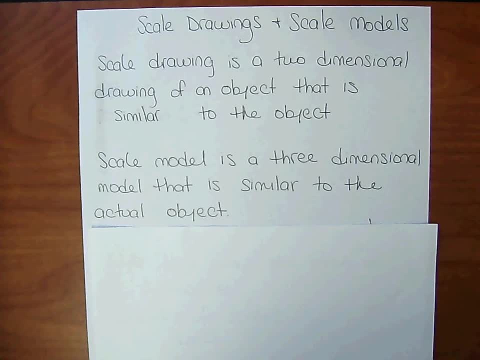 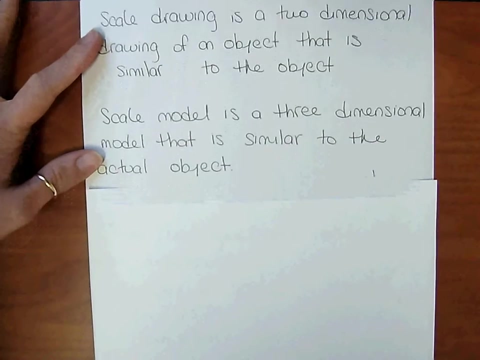 have the same shape, different size And, in order for figures to be similar, the corresponding angles are congruent and the corresponding sides form a proportion. When you have a scale drawing or a scale model, you have a scale or a key and it gives the ratio of the dimensions. 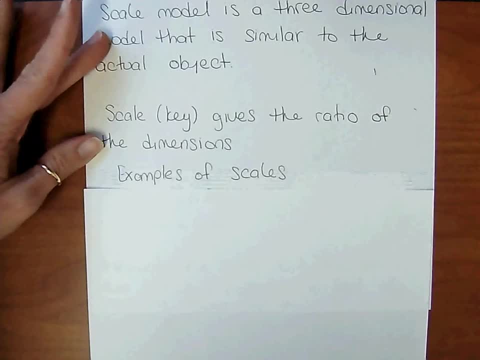 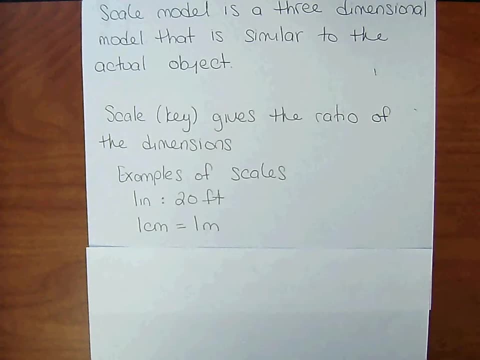 Here are some examples of scales: One inch to 20 feet. one centimeter equals one meter. These are not facts of life. We know that one inch is not the same as 20 feet, but in this drawing or in this model, 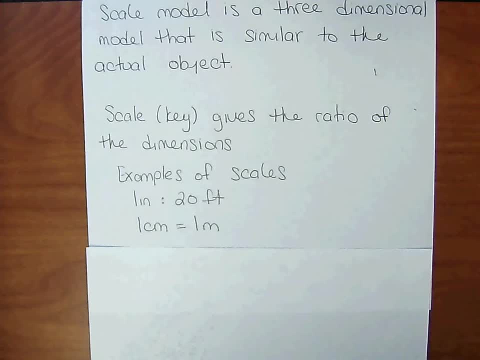 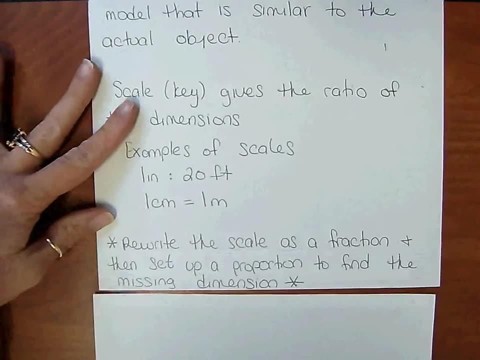 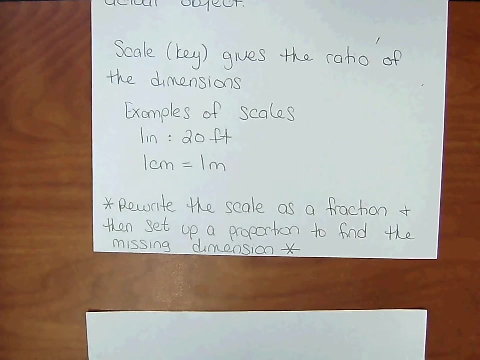 one inch to 20 feet is the fact, and you're going to treat it as such while you're working out the problem. So what you want to do is rewrite the scale as a fraction and then set up a proportion to find the missing dimension. 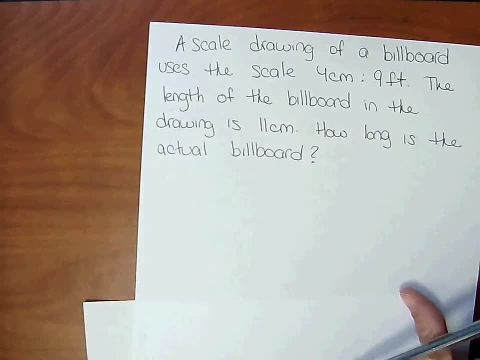 So a scale drawing is a two-dimensional model. A scale drawing is a three-dimensional model. We know that one inch is not the same as 20 feet, but in this drawing or in this model, one inch is four centimeters. 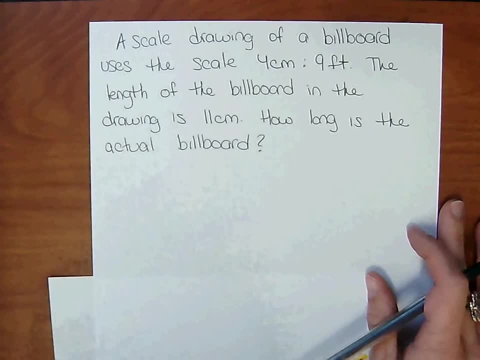 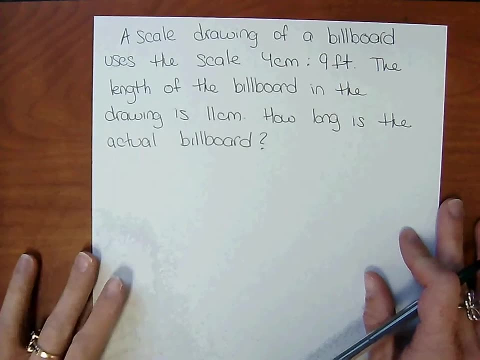 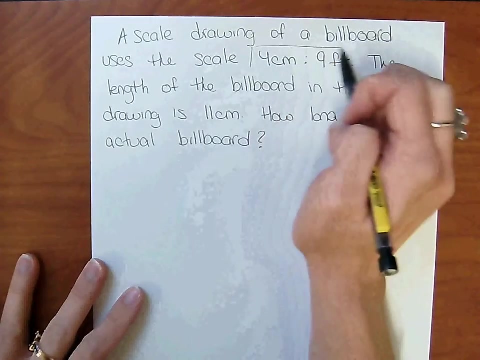 The length of a drawing of a billboard uses the scale four centimeters to nine feet. The length of a billboard in the drawing is 11 centimeters. How long is the actual billboard? Start with the fact or the scale: Four centimeters is equal to nine feet. 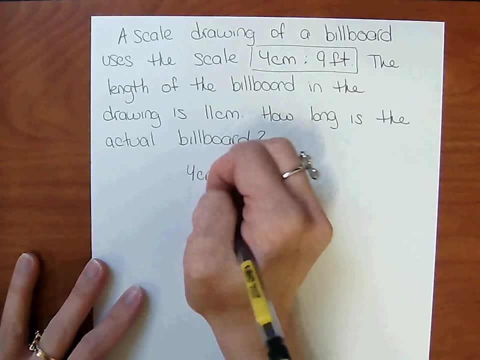 So we're going to set up a proportion: Four centimeters nine feet equals. Well, we were given. So let's go back and I'm going to turn on the machine. I'm going to take aÉ. I'm going to take a look at this. 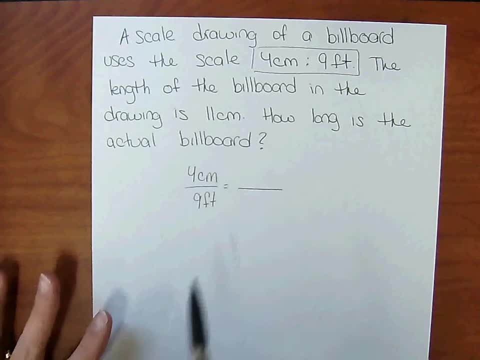 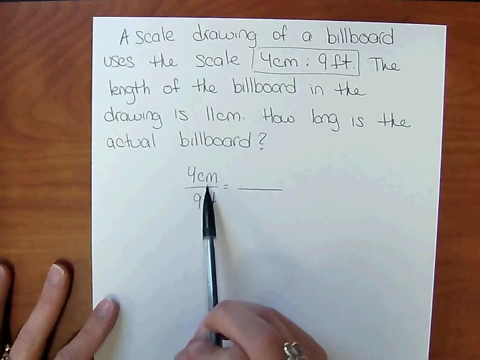 given that the length of the billboard in the drawing is 11 centimeters, so we're going to line up our units. Centimeters are going to line up with centimeters, so we have them in the numerator. So we're going to put 11 centimeters in the numerator and then x in. 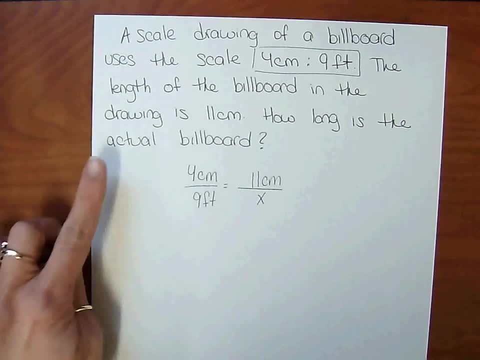 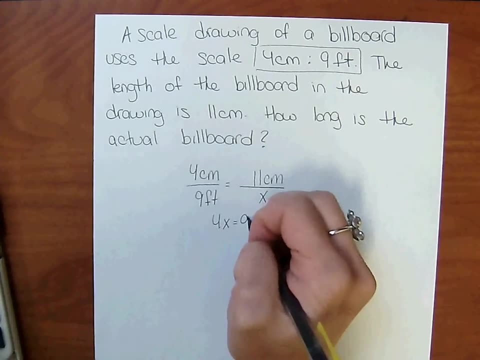 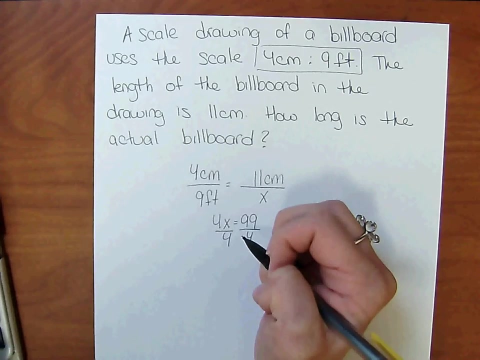 the denominator, because we're trying to find the actual billboard and the actual length will be in feet. So cross multiply 4x equals 99.. Solve for x, Divide 4 on both sides, And x equals 24.75 feet.